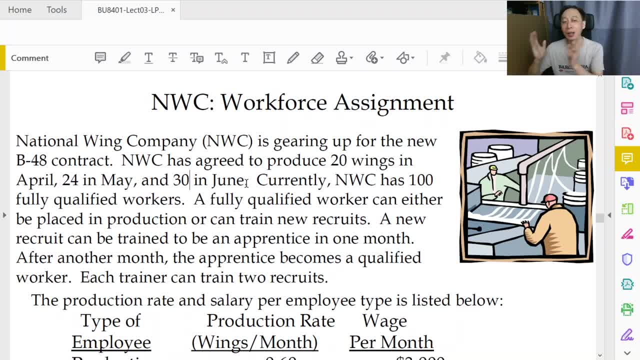 order. so this one produce 20, the next month produce 24 and the third month produce 30. make to order, finish. there's no, no way to optimize, but let's see what. what happens? it has workers right. so you have 100 fully qualified workers and we. 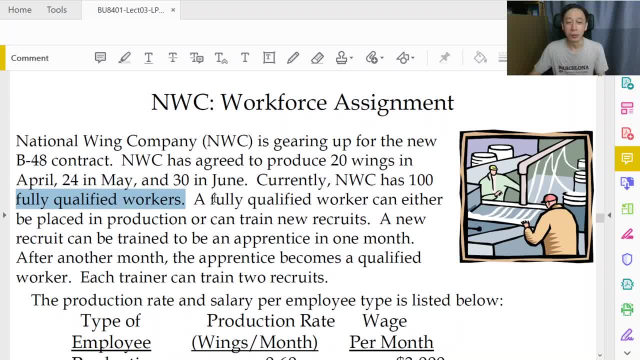 might wonder at this point: what does fully qualified mean? so let's read on. so a fully qualified worker can either be in production or in training. ah, okay, so when this situation where we can grow, we can train new recruits, their incoming workforce, a new recruit can be trained to be an apprentice in a month, one month. 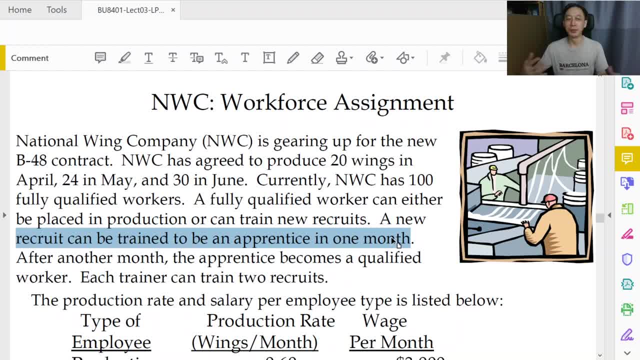 right. so now notice how this looks so different from the financial application example we discussed earlier on. yet yet, if you think about it, if we rephrase it, it's saying that this recruit sounding like an investment option, right? this investment option takes one month to mature. this recruit takes one month to. 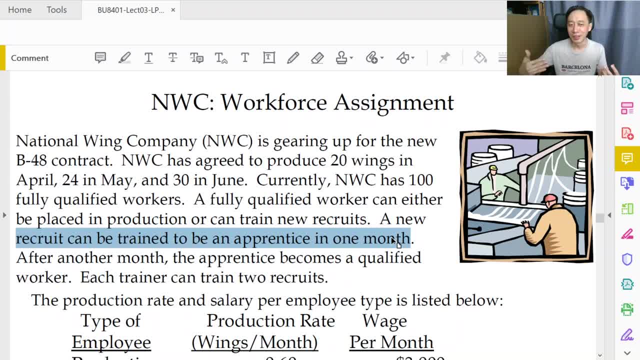 mature into the status called apprentice. if you think about it this way, then as far as translation into LP model and constraints are concerned, then the same right, because maturity in financial applications is basically changing or promotion, change of status in the operations situation or human resources duration right. so for that matter they 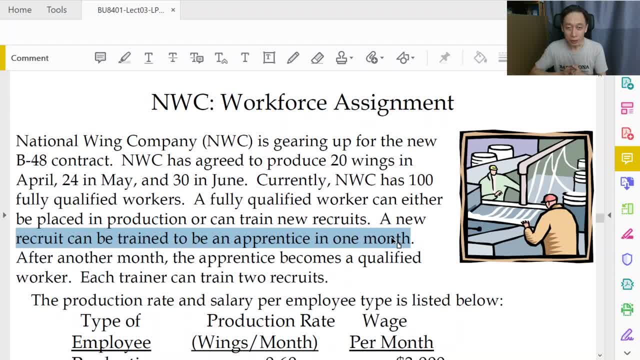 are the same when it comes to translation, so let's keep that in mind. although it sounds like very new- our first discussion of promotion or or a change of status after a training period- this is just like an investment maturing in a given duration. right, it's the same. and we know how to model time in lp model now, so we can reuse our 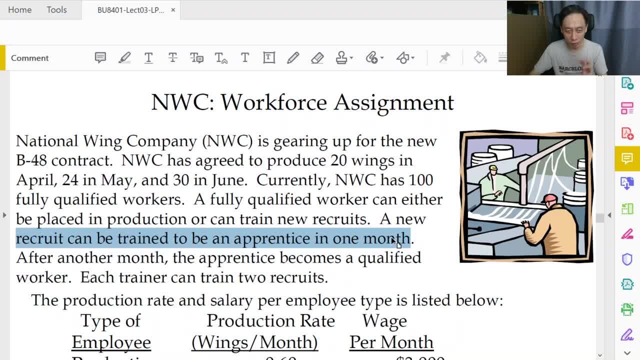 tricks there. nothing extremely new here, although the wordings are very different. the, the uh application domain is sounding very different. but from the lp modeling and translation perspective, same trick. right after another month. that means uh for starting from as an apprentice. it takes another month for the apprentice to become a worker, at which point 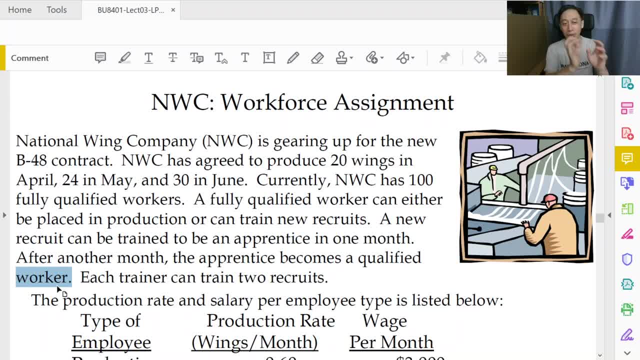 this qualified worker can either be deployed as production or as trainer. each trainer can train at most two recruits. just to take care of the case that there are, there are odd number of recruits, right? so each trainer can train up to two recruits, because the apprentice, they, they, uh, the attention has to be there. so 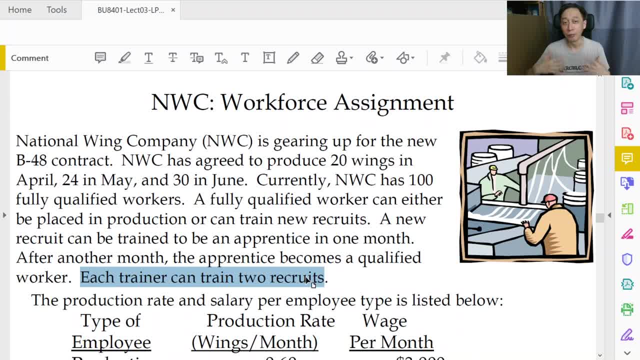 say the company policy says each trainer can cannot take care of more than two recruits, sounds reasonable, and it is this part, it is this part that we will encounter some difficulty. so, uh, i will focus on this line in a while, but let's, let's quickly scan through the rest. 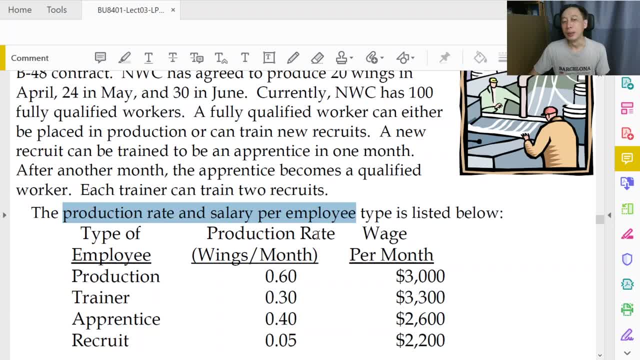 we are given production rate salary and, uh, we can imagine these will be the coefficients that we need to plug into the lp model and we can imagine these will be the coefficients that we need to plug into. uh, just take one look, and it has to be constraints because it's probably 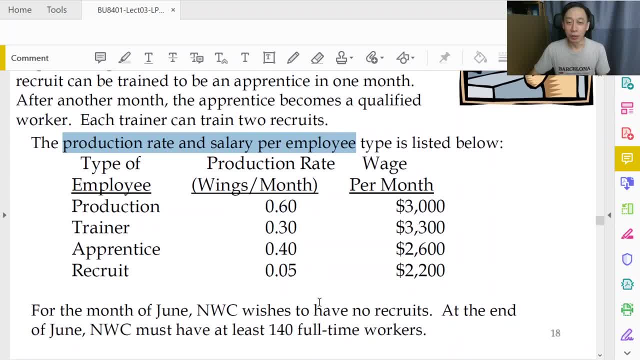 uh, constraints, coefficients, right. of course it can also be numbers that we plug into objective function. but let's see what do we have to optimize, don't assume. let's see what we need to do. in this case, for the month of june, nwc wishes to have no recruits. at the end of june, nwc must have at least. 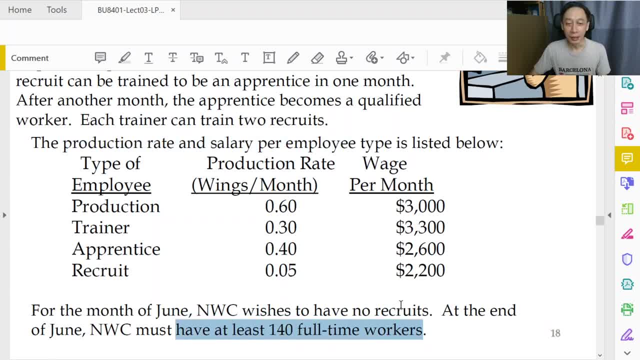 time workers now notice how this, this sentence sounds like the finance show application case, where we say: at the end of the four month planning horizon, we must have at least 10 million dollars. here it is at the end of, uh, the three month planning horizon, we must have at least 140 workers. 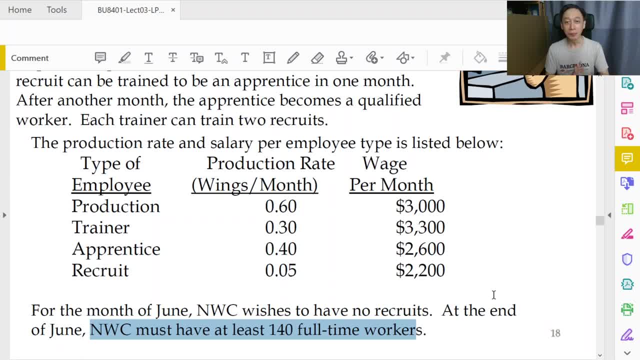 okay, fine, one is money, one's worker, but let's say amount of dollars and number, quantity of workers: at least 10 million, at least 140. same translation, right, so we can do the same thing. and it involves month, and when it involves months, we need to be. 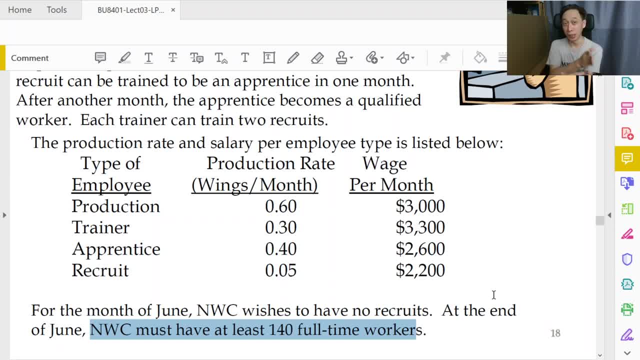 careful of the quantity that we snapshot within the month. is it at the end, the middle, the end, right? so again, we want to be extremely clear with our definition of the decision variables. uh, at what point in time of the month are we counting? yeah, because the numbers can change. so 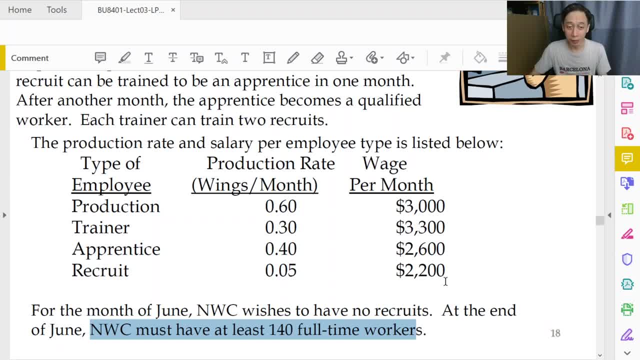 again, we default to using start of the month or start of the of the intervals. if it's week of planning, then we say at the start of the week or at the start of the year. so here we say at the start of the month. now, um, we're given the production rates for each kind of workers: production produce. 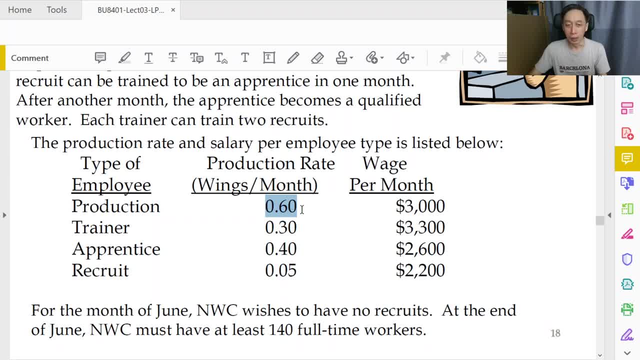 workers produce a a lot uh, 0.6 of a wing per month very, very rapidly. trainer half the rate, but trainer gets to train people so we allow for half time. trainer gets paid a lot more uh and production 3 000 right. so apprentice turns out to be um, contributing more to the progress of wings. 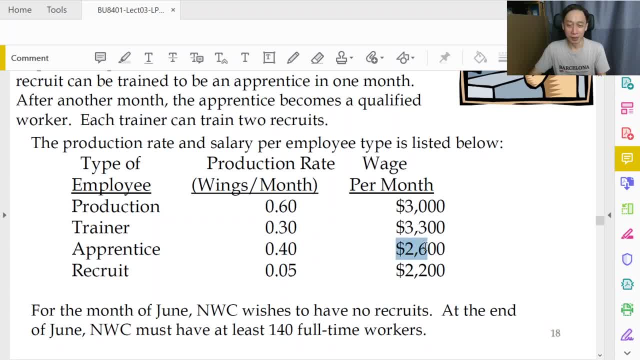 production than trainer. equally decently, and we need to get up to speed of for recruits because they contribute 0.05. maybe they help to carry tools, maybe they buy lunch for the workers and therefore improve productivity of the workers, someone. so they contribute in that sense and they are paid a salary. okay, now perhaps in 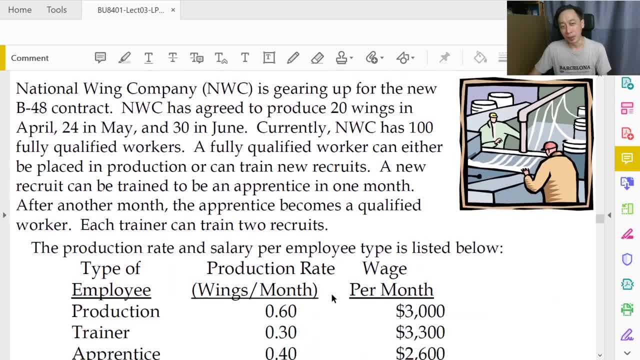 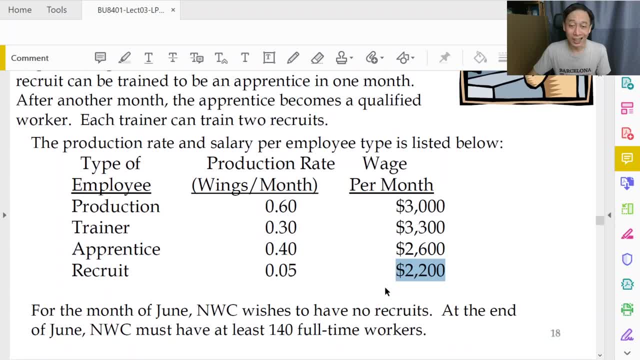 this summary slide. it wasn't stated as in what is the concern of the problem owner. but of course we should be able to guess- although it's not ideal, we shouldn't be guessing- but we can deduce that saving cost should be the prime objective of this company, this company's operations. it is possible that we also 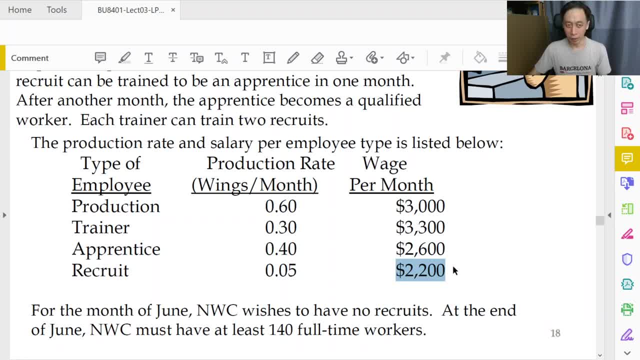 want we may also to maximize, you know, progress of the wings, or maximize the number of trainers for a certain month, or maximize certain number of production workers for a certain month, although those the the real goal or reasons to have those objective functions might not be so clear. so for operations typically it is: 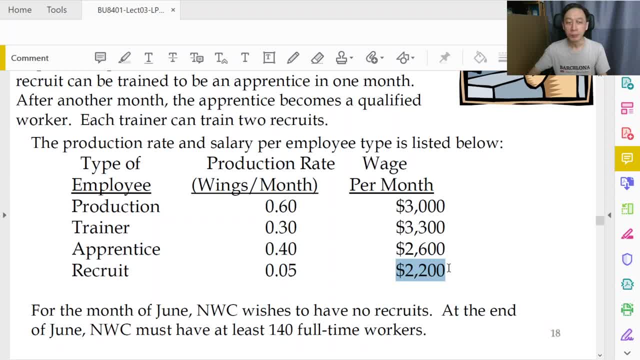 to minimize overall costs. okay, so let's see how we can do that. clearly, we need to have four decision variables already: number of number of production workers. number of trainers, number of apprentice. number of recruits. the question is also: how many recruits do we hire? three take in at the start of 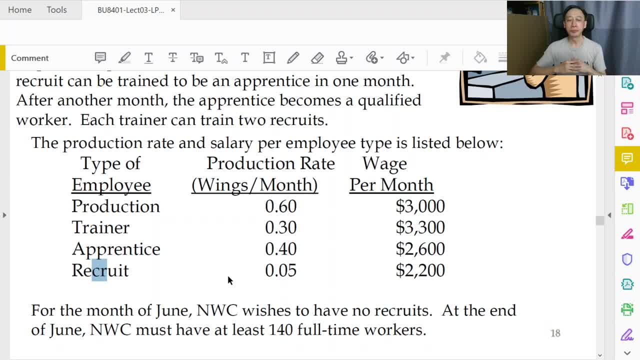 every month, remember right, so we not only have to have four variables, because then we say, well, we have three months to think about right, ever. Every month we ask how many worker of each of the four types do we need? Of course, the second month's production workers is not totally delinked from the previous. 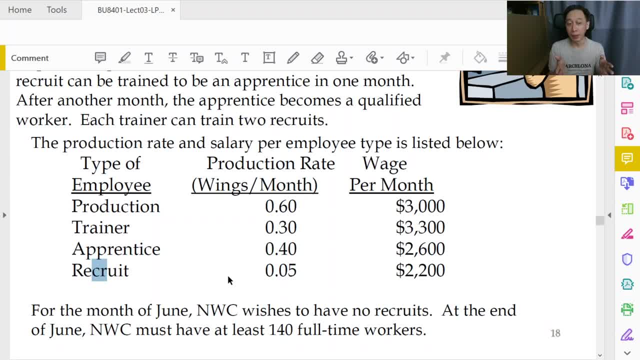 month's production workers. The second month's apprentice is not completely detached from the previous month's recruit because it takes one month to mature to get promoted to apprentice. So we need to link them together, but instead of using the subtractive way of saying things. 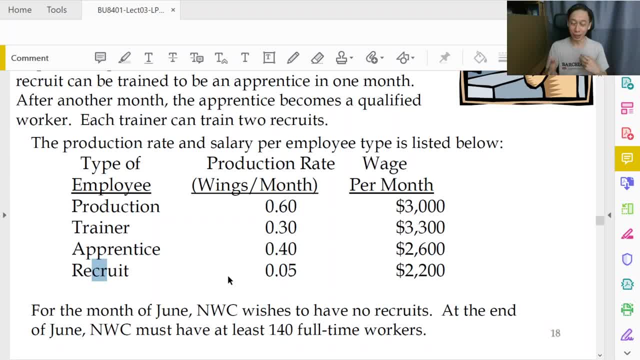 given that the second month has five apprentice and 10 trainers and 10 production workers and a total of 30 workers, then we minus, minus, minus to get the number of recruits. We don't deduce the number. Okay, We don't subtract to get the results. 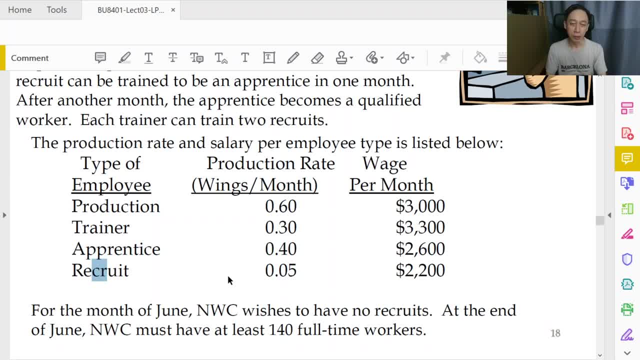 Instead, we dedicate fresh decision variables to describe each kind of unknowns that we have. And then, when we need to describe the aggregate, for example, we ask: total number of workers must be at least 140.. Then we add up the individual component variables to come up with aggregate total. 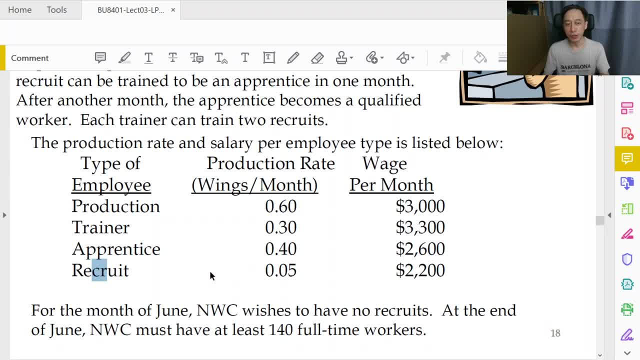 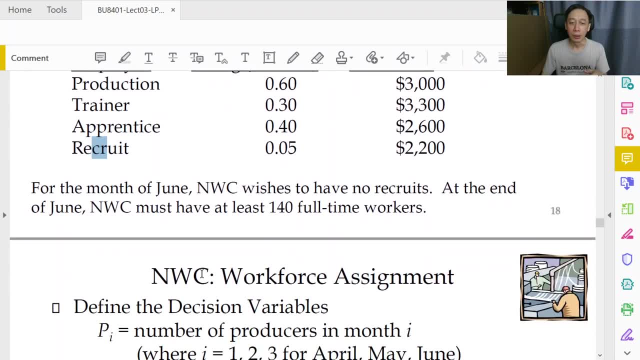 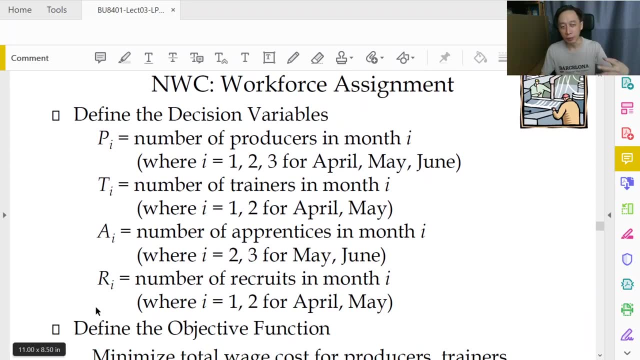 So, very quickly, we are going to basically flesh out four. So we have an aggregate total of four, four months, three months and twelve decision variables. So let's take a look at the offered solution here. So indeed, we have four types of counts of different four kinds of workers for each of. 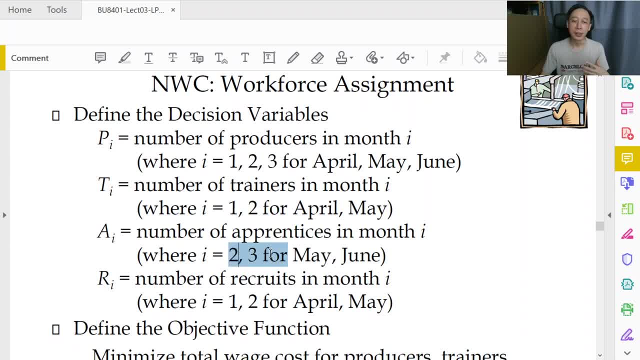 the months. That's the basic idea, basic thinking. But we know that, for example, at the start of the third month we will not be hiring Right. So in June we will not be hiring. So we can start the third month. 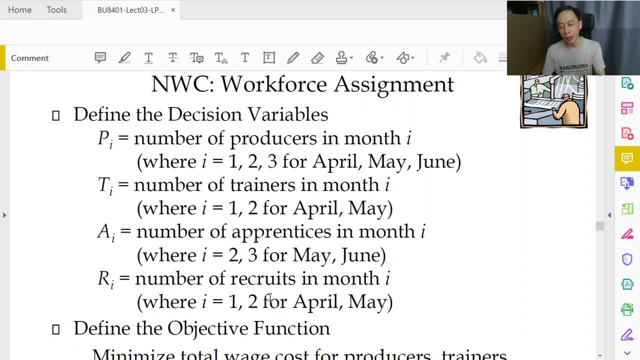 So we can start the third month. We know that One way is to say we have R3 for June and then constrain it: set R3 to be equal to 0. But that's sounding a little bit strange because we already know the outcome. 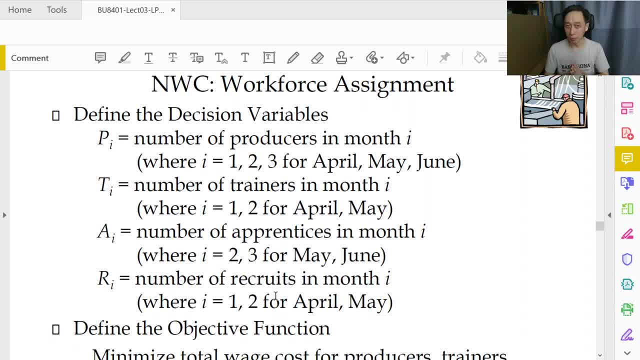 We cannot optimize it. Company policy says R3 equals to 0. So we can say R3, define R3, and constrain it to be 0. But since we already know the outcome, we can just delete the variable. So there's no 3, R3 for June. 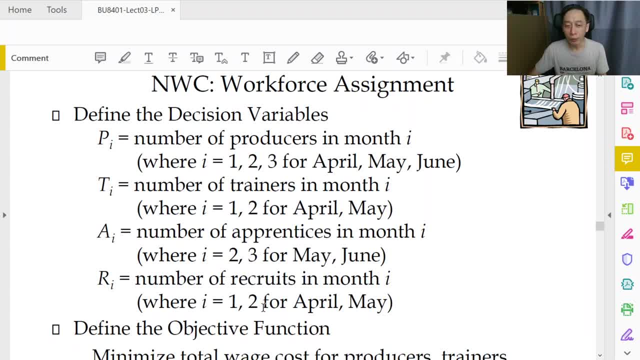 If there is no R3 for June, then we also don't need trainers for June. So for that reason we sort of optimize the model a little bit by saying that, okay, we already know by the logic of the company's policies. 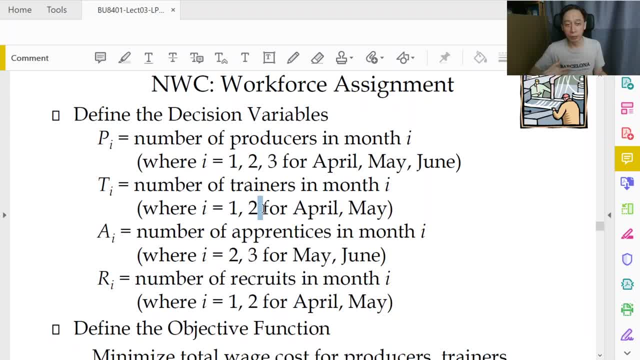 we need trainers to train recruits to become apprentices. If there are no recruits, we don't have to allocate trainers, Or we pretend We don't know how many trainers we need and then let model figure out that it should be 0.. 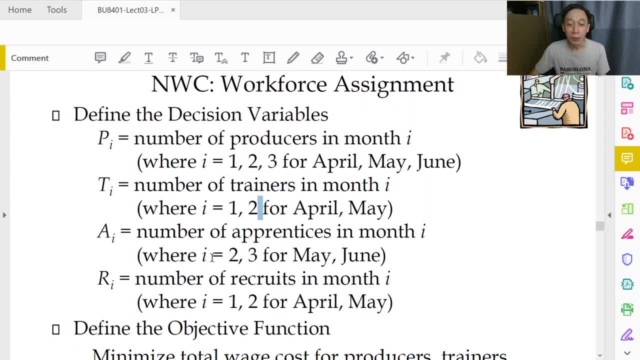 We don't need that, so we cancel out T3.. Now, for first month there should be no apprentice, because we currently don't have any recruits. So when we hire recruits they cannot be directly promoted to apprentice. So even if they're very experienced, very seasoned, they come in as recruits. 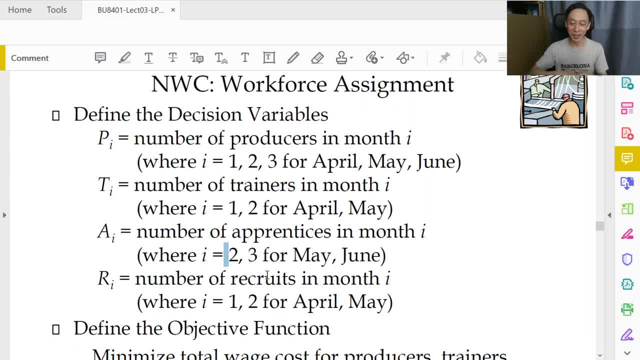 Now you wouldn't enjoy that if you are a seasoned college graduate Who can be given exam credits to jump into university second year, right, So that's exemption. but they don't have exemptions. They all come in as recruits and they take one month to get promoted.